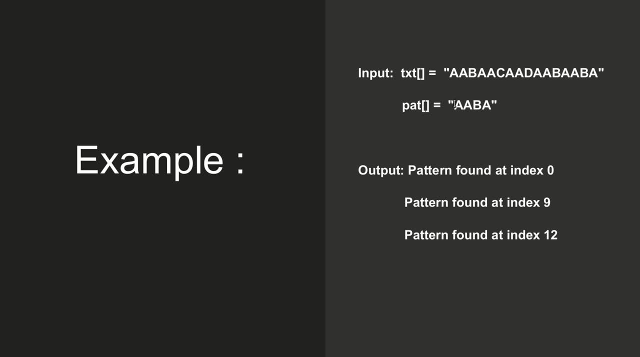 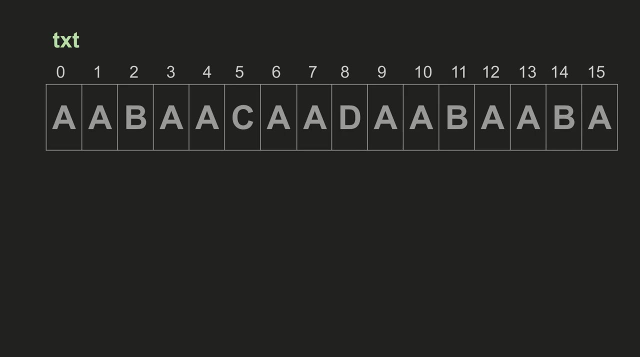 in text string where the pattern string is found, like aapa is found starting from index 0 of text string, then starting from index 9. and then starting from index 12.. So this should be printed in our output. So if I have text string of size 16, 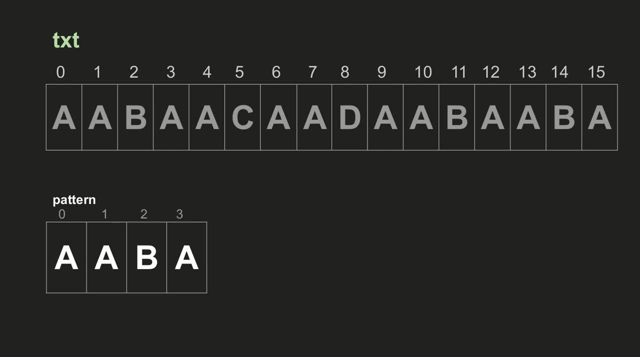 and pattern string of size 4, then I need to take a window size of 4, which is the size of pattern string. Now we start running the window over the text string starting from index 0. This is the window in text string. then we compare this window with the pattern string. 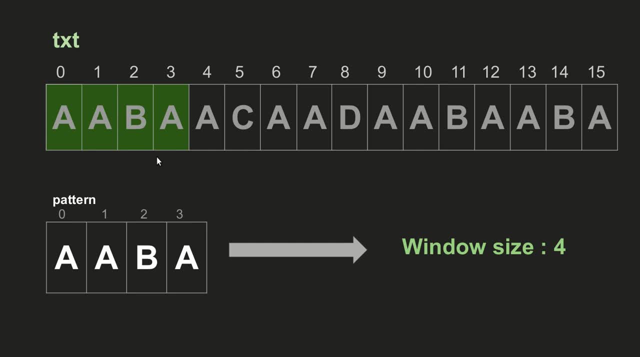 and if both these strings are found to be equal, then we say that the pattern has been found at that particular index in text string. Then we move the window forward and again compare the window with the pattern string. Similarly we keep moving the window until we reach to the last window. 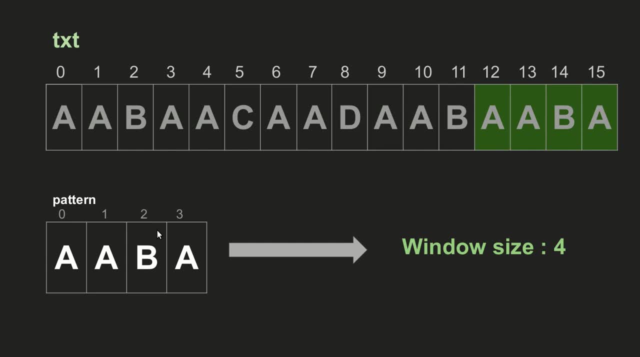 Then we move the window forward and this is the last window in text string. So we see that if text string size is 16 and the pattern string size is 4, then the last index where the window should be there is given by 16-4, that is 12.. 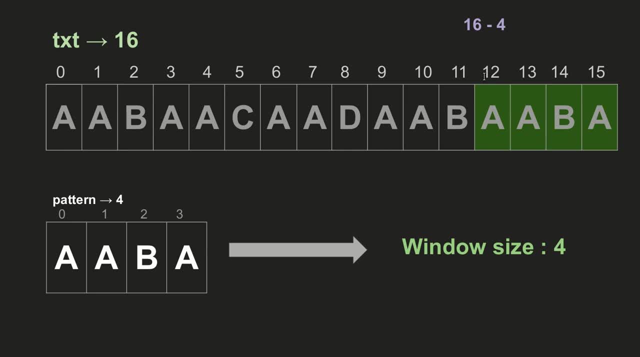 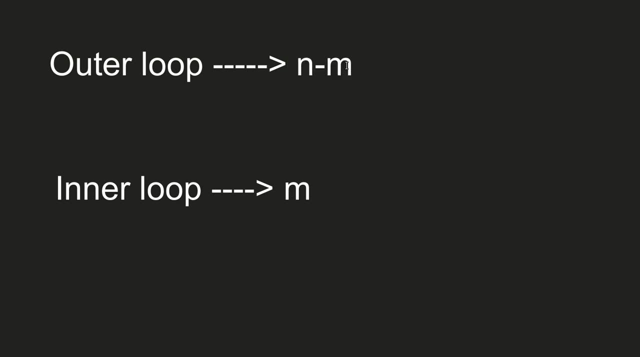 So the window runs from 0 to 12.. So there should be an outer loop in the code which runs for n-m time. This indicates the starting index of the window. n is size of the text string and m is size of the pattern string. 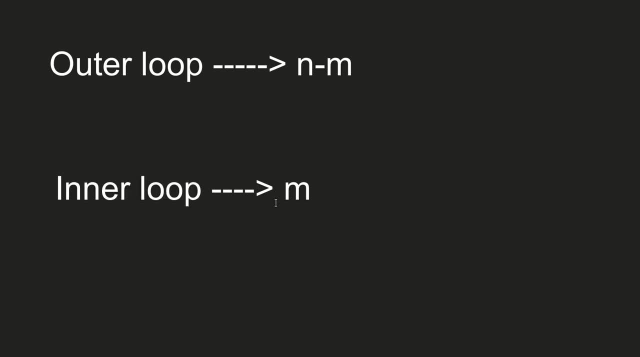 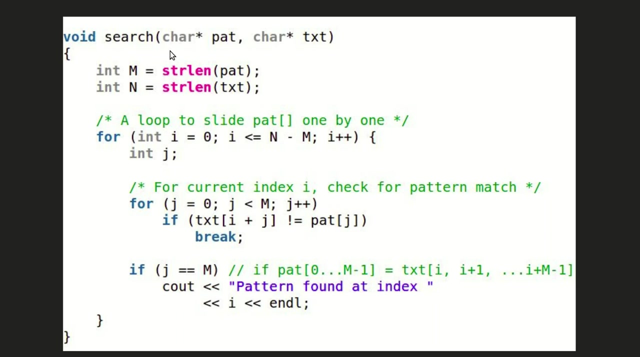 Then, for each window, there is an inner loop which runs from 0 to m- that is the size of the pattern string- and then compares the window with the pattern. Coming on to the code, this code is taken from GeeksforGeeks. The search function takes as input: 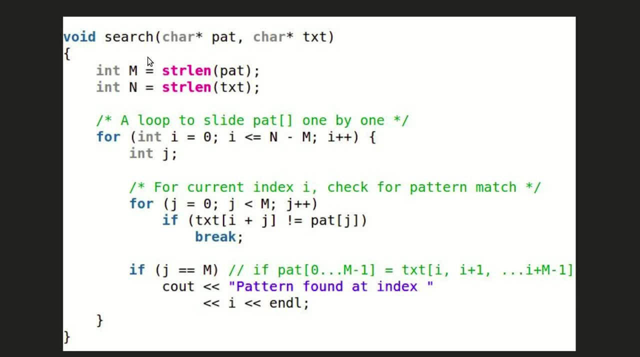 the text and pattern string and then computes and stores their length in m and n. Then there is an outer loop from 0 till less than equals to n-m, which represents the window starting index. Then for each window there is an inner loop which runs from 0 till less than m.